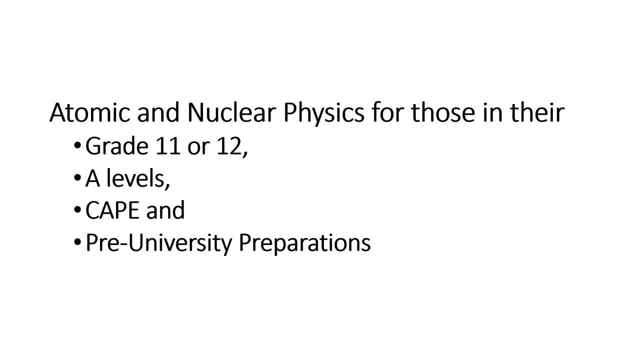 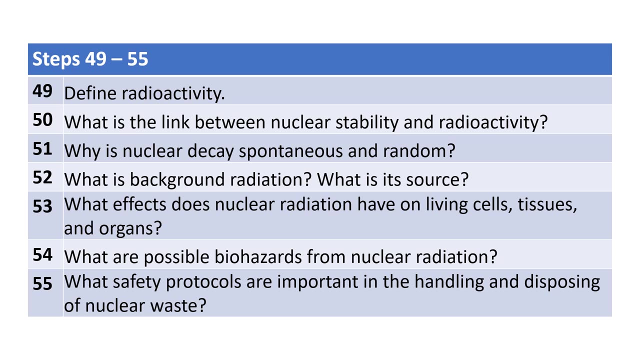 Atomic and Nuclear Physics for those in their grade 11 or 12, A-Levels, CAPE and Pre-University Preparations. Steps 49 to 55.. 49. Define Radioactivity. 50. What is the link between Nuclear Stability and Radioactivity? 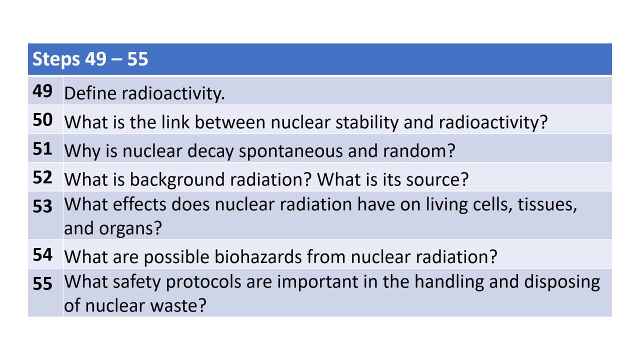 51. Why is Nuclear Decay spontaneous and random? 52. What is Background Radiation? What is its source? 53. What effects does Nuclear Radiation have on living cells, tissues and organs? 54. What are possible biohazards from Nuclear Radiation? 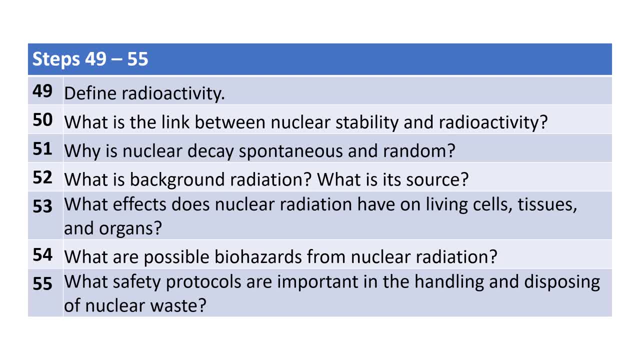 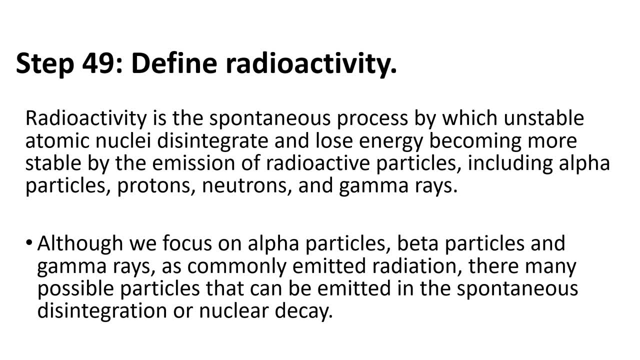 55. What safety protocols are important in the handling and disposing of nuclear waste? Step 49. Define Radioactivity. Radioactivity is the spontaneous process by which unstable atomic nuclei disintegrate and lose energy, becoming more stable by the emission of radioactive particles. 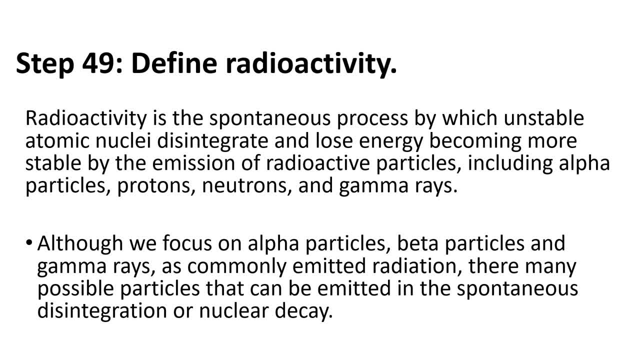 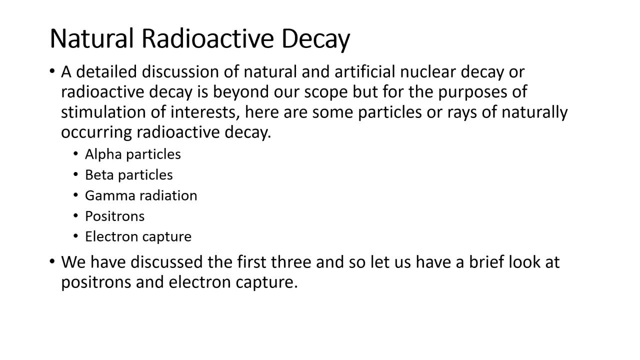 including alpha particles, protons, neutrons and gamma rays. Although we focus on alpha particles, beta particles and gamma rays as commonly emitted radiation, there are many possible particles that can be emitted in the spontaneous disintegration or nuclear decay. Natural Radioactive Decay. 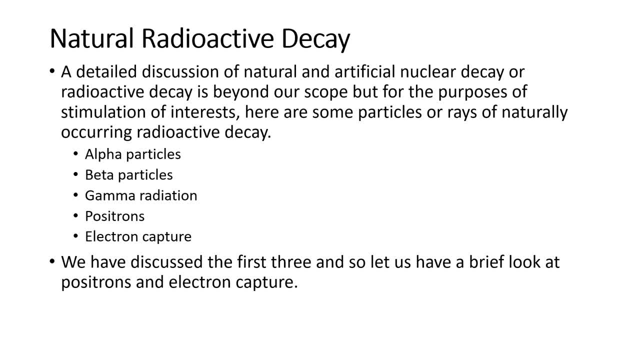 A detailed discussion of natural and radioactive decay is available on our website. A detailed discussion of natural and artificial nuclear decay or radioactive decay is beyond our scope, but for the purposes of stimulation of interests, here are some particles or rays of naturally occurring radioactive decay. 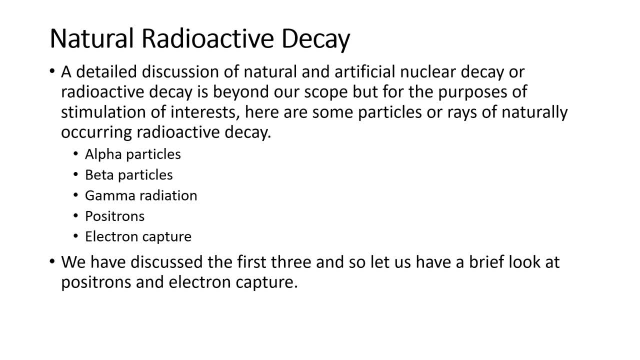 1. Alpha particles, 2. Beta particles, 3. Gamma radiation, 4. Positrons, 5. Electron capture. We have discussed the first three, and so let us have a brief look at positrons and electron capture. 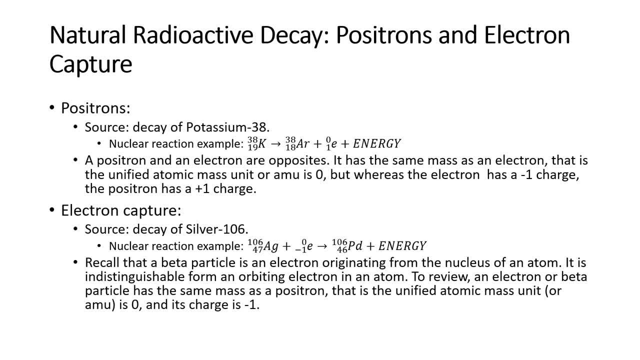 Natural Radioactive Decay, Positrons and Electron Capture. One positron source is the decay of potassium-38. Nuclear reaction example: K38, 19 decaying to a 38, 18 plus an electron. 0 negative 1 plus energy. 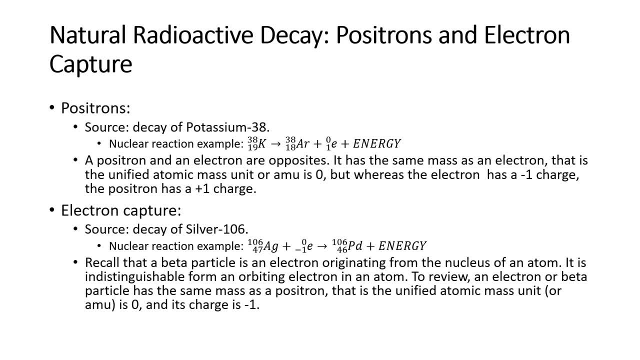 A positron and an electron are opposites. It has the same mass as an electron, that is, the unified atomic mass unit, or AMU, is 0,. but whereas the electron has a minus 1 charge, the positron has a plus 1 charge. 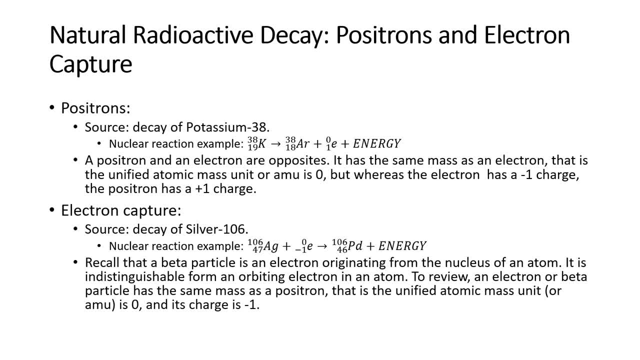 Electron capture is observed in the case where the nucleus of silver 106-47 receives an electron to become lead 106-46.. Recall that a beta particle is an electron originating from the nucleus of an atom. It is indistinguishable form an orbiting electron in an atom. 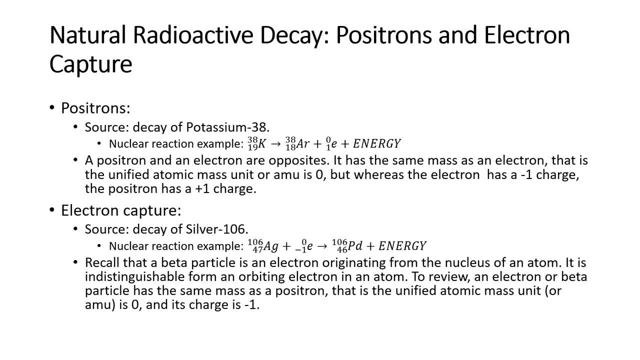 To review. an electron or beta particle has the same mass as a positron, that is, the unified atomic mass unit, Or AMU, is 0 and its charge is negative 1.. Step 50.. What is the link between nuclear stability and radioactivity? 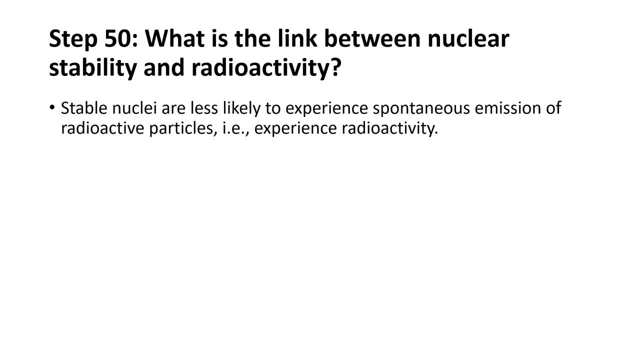 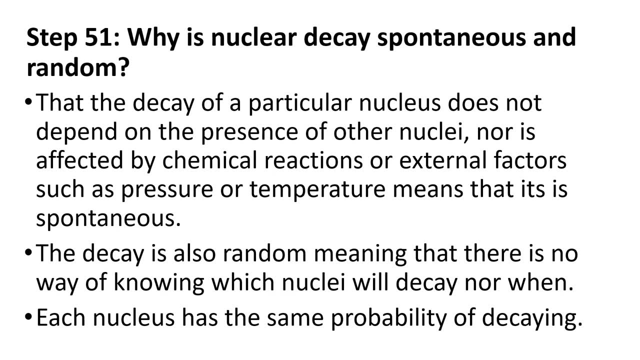 Stable nuclei are less likely to experience spontaneous emission of radioactive particles, that is, experience radioactivity. Step 51.. Why is nuclear decay spontaneous and random? That the decay of a particular nucleus does not depend on the presence of other nuclei, Nor is affected by chemical reactions or external factors such as pressure or temperature, means that it is spontaneous. 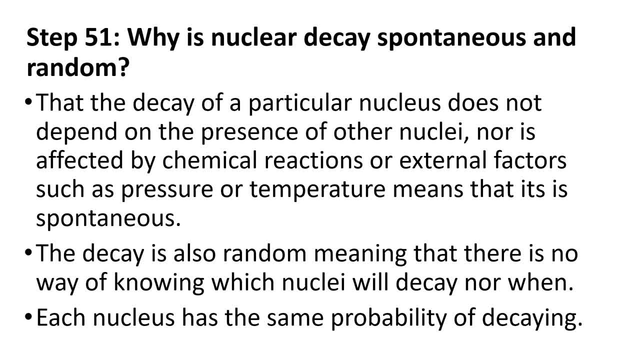 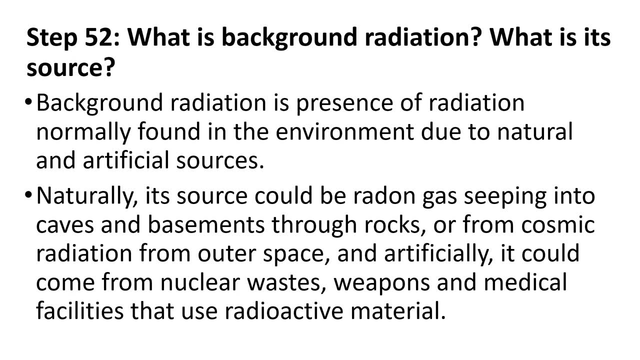 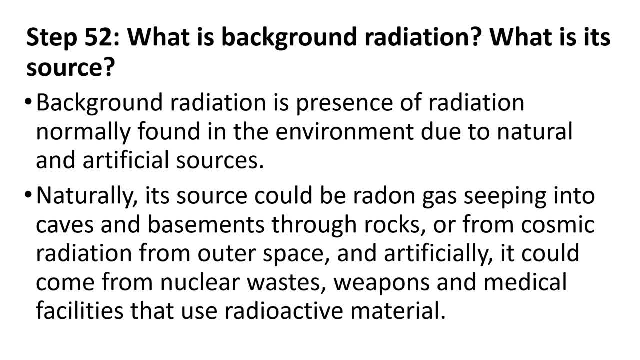 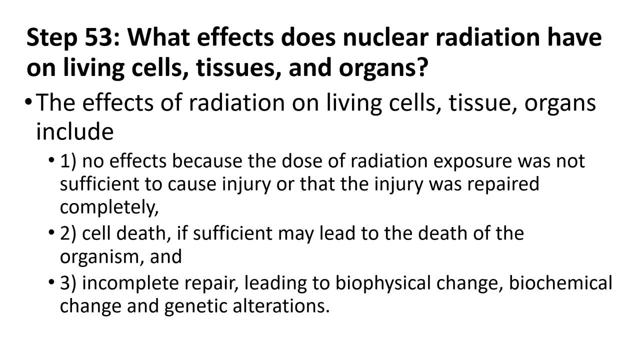 Naturally, its source could be radon gas seeping into caves and basements through rocks, or from cosmic radiation from outer space, and artificially it could come from nuclear wastes, weapons and medical facilities that use radioactive material. Step 53.. What effects does nuclear radiation have on living cells, tissues and organs? 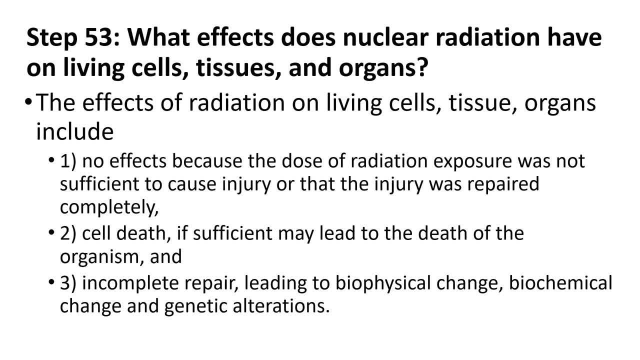 The effects of radiation on living cells, tissue organs include: 1. No effects because: 1. No effects because dose of radiation exposure was not sufficient to cause injury or that the injury was repaired completely. two: cell death, if sufficient, may lead to the death of the organism, and three- incomplete.